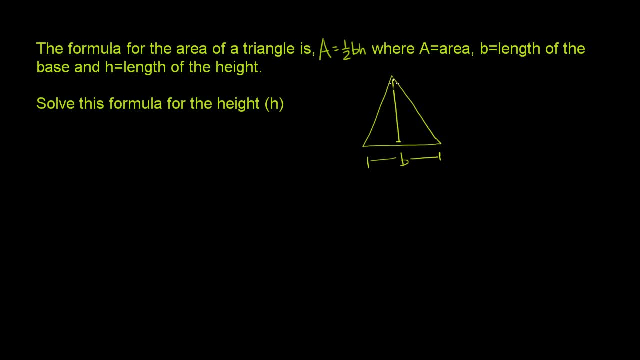 And then this distance right here is our height, That is the height of the triangle. Let me do that in lowercase h because that's how we wrote it in the formula. Now they want us to solve this formula for the height. So the formula is: area is equal to 1 half base times height. 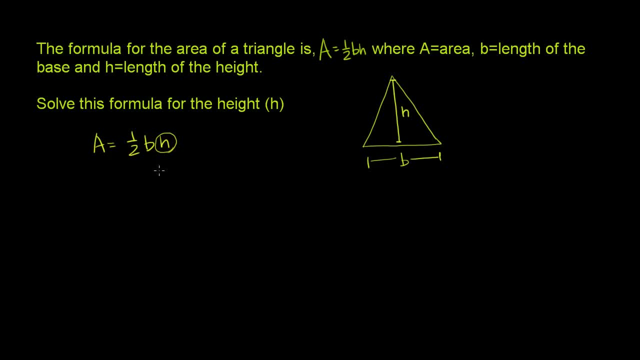 And we want to solve for h. We essentially want to isolate the h on one side of the equation. It's already on the right-hand side, So let's get rid of that. Let's get rid of everything else on the right-hand side. 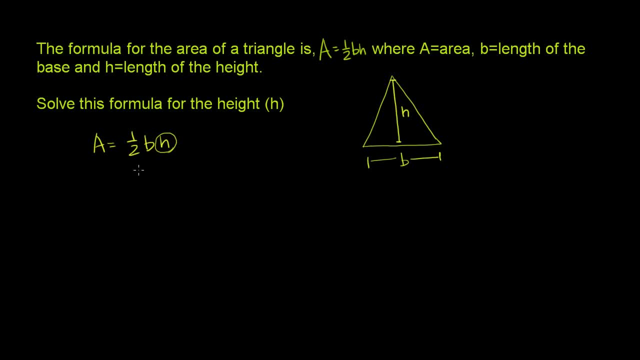 So we could do it. well, I'll do it one step at a time. We could kind of skip steps if we wanted to, But let's see if we can get rid of this 1 half. So the best way to get rid of a 1 half- and it's being multiplied by h- 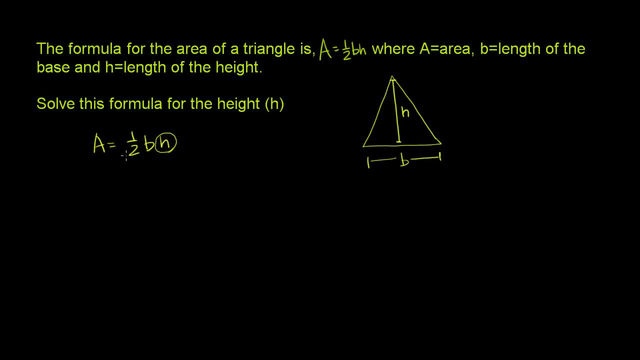 is if we multiply both sides of the equation by its reciprocal, If we multiply both sides of the equation by 2 over 1, or by 2.. So let's do that, So let's multiply. Remember anything you do to one side of the equation. 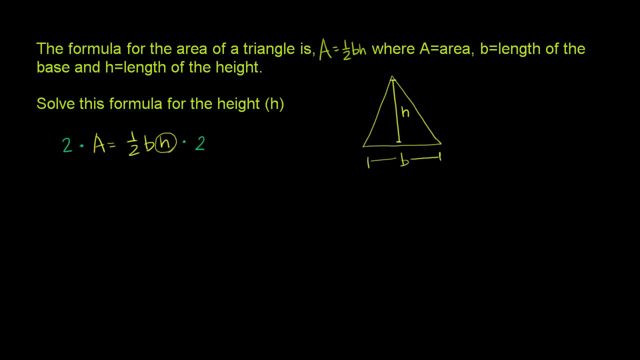 you also have to do to the other side of the equation. Now, what did this do? Well, the whole point behind this is the whole point behind: multiplying by 2 is 2 times 1, half is 1.. So on the right-hand side of the equation, 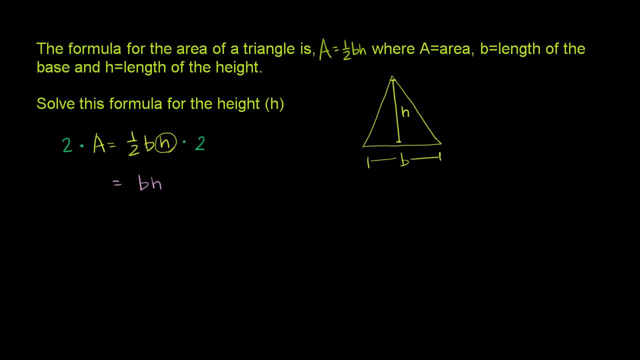 we're just going to have a bh And on the left-hand side of the equation we have a 2a And we're almost there. We have a b multiplying by an h. If we want to just isolate the h, we 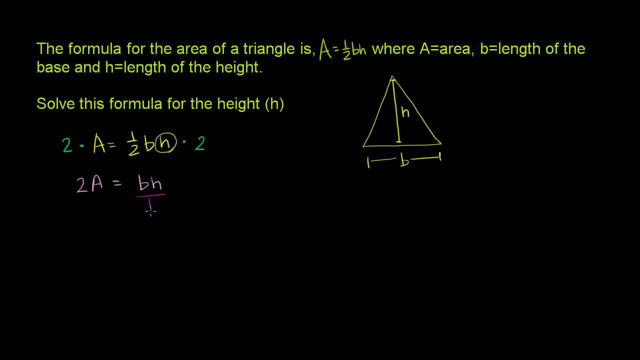 could divide both sides of this equation by b. We're just dividing both sides. You could almost view b as the coefficient on the h. We're just dividing both sides by b. And then what do we get? Well, the right-hand side, the b's cancel out. 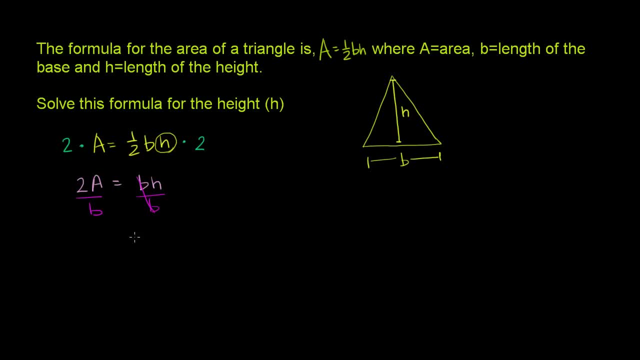 And the left-hand side. we're just left with 2a over b, So we get h And I'm just swapping the sides here. h is equal to 2a over b And we're done. We have solved this formula for the height. 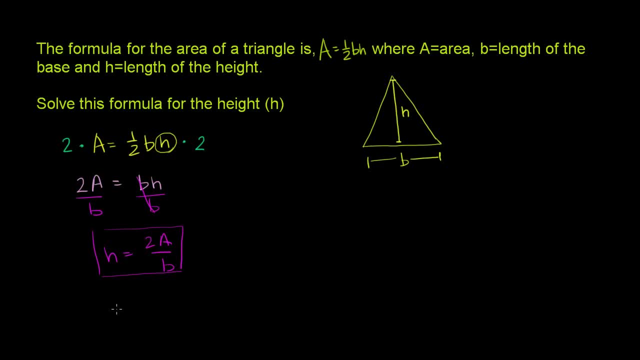 And I guess this could be useful. if someone just gave you a bunch of areas and a bunch of base lengths and they said: keep giving me the height for those values or for those triangles.